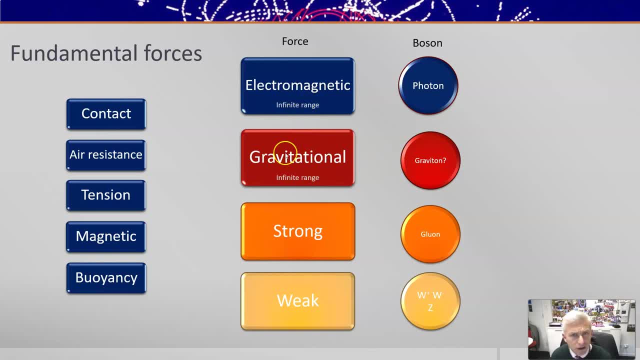 hypothesized to exist. these two forces have infinite range. gravitational forces act across the universe, but obviously the closer you are, the bigger they are, whereas the strong and weak force only act within the nucleus. you can think of bosons, like exchanging footballs between two players on roller skates. if 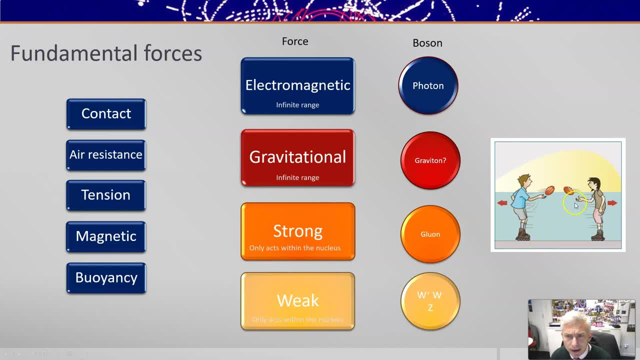 they threw a ball between each other, they would exert a force on each other and repel each other. now, this is only an analogy. it is not exactly what's happening. it is certainly not a force when they exchange momentum, but it is an analogy to think about how it works. of course, photons can also attract two. 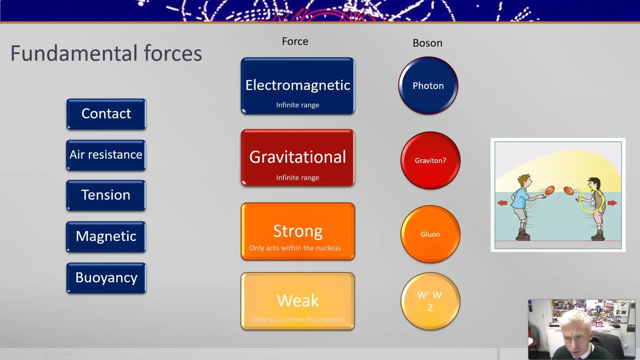 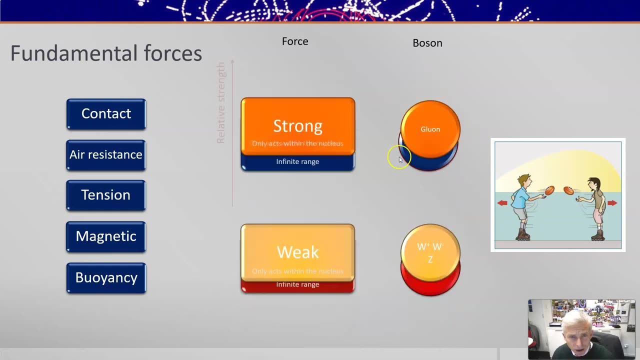 objects, a positive and a negative charge, object exchange, a virtual photon and they draw, drag each other together. so the analogy doesn't work there. you'd have to imagine throwing antimatter particles or something else weird, or perhaps grabbing each other's particles and pulling the things things together if we sort these into order of relative. 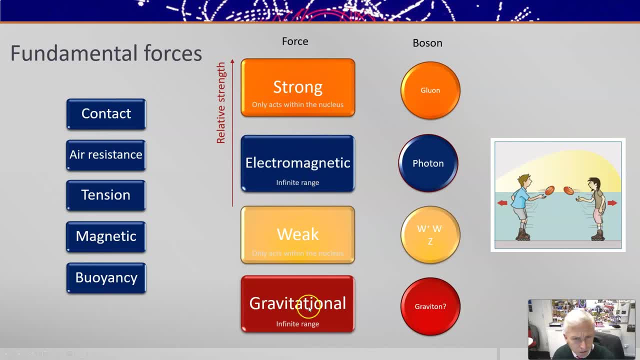 strength, then the strong force, predictably, is at the top and the gravitational force is at the bottom. if you were to jump out of a window, gravitational force would not hurt you. it will accelerate you very slowly as you get towards the ground and you would speed up, sure, but the thing that hurts you is the 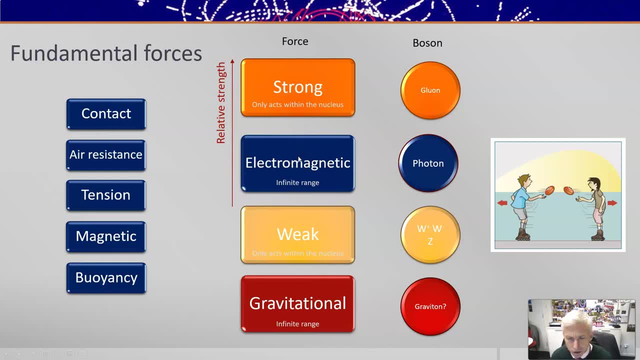 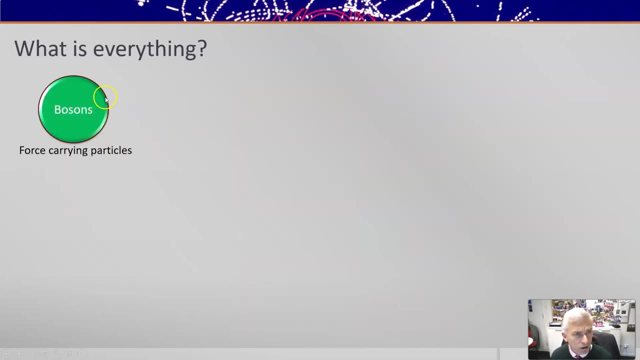 electromagnetic force. when the electrons in your body are repelled by the electrons on the floor, the strong force is even stronger than that and it only acts inside the nucleus to bind the nucleons together. so what is everything? well, everything in the world consists of bosons in the universe and particles of 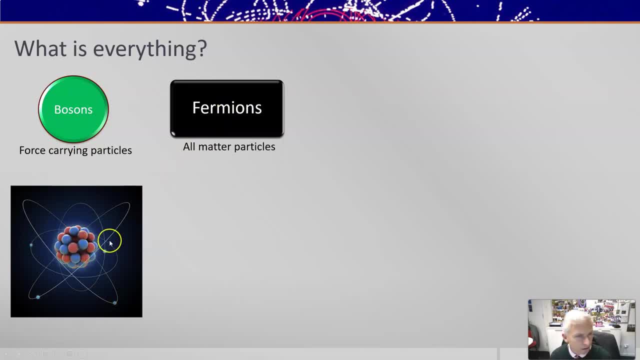 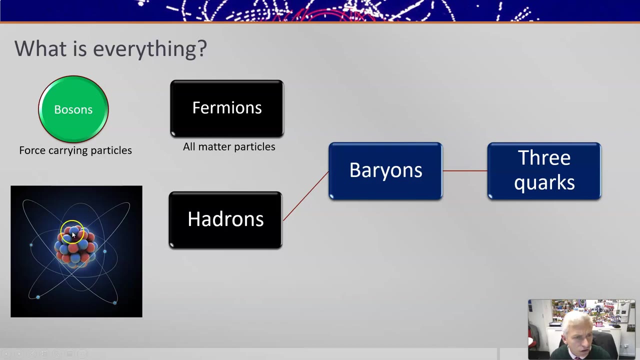 matter, fermions. so all of these particles are particles of matter, and the heavy ones upon ones, in the nucleus for example, are called hadrons. hadron just means heavy, and a Hadron can be a baryon, and a baryon consists of three quarks, so the protons and the neutrons are all baryons, and it can also be mesons. 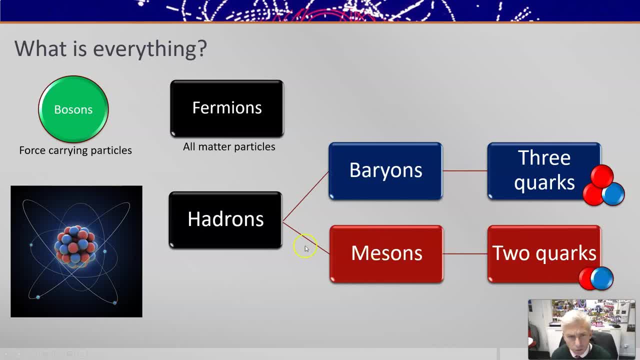 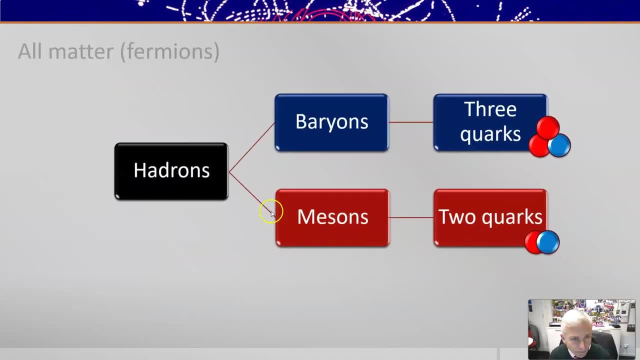 mesons are two quarks. pairs of quarks exist in strange formations and we don't see many of them in the universe very often. but they do exist and it is important to know how they work. so fermions, hadrons and the neutrons are called"hadrons'. 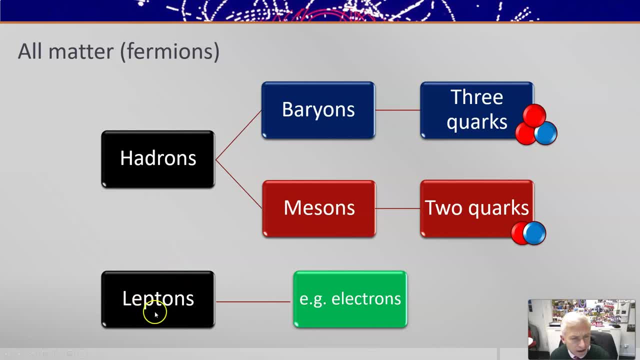 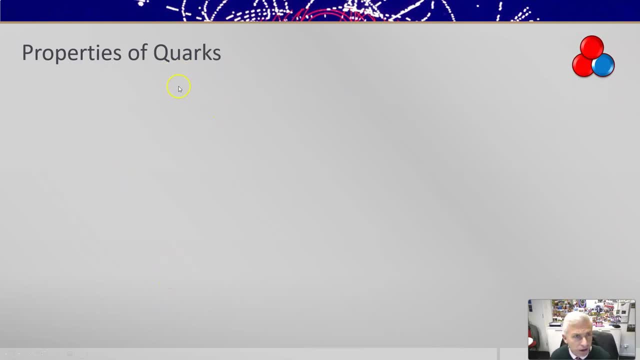 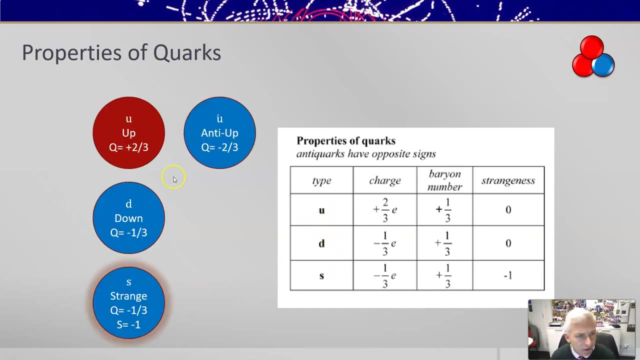 electrons and leptons. leptons are light particles, light in mass. electrons are leptons. so those are all the matter particles and we'll show you a bit more in a second. so quarks: we've got three quarks in this table, here and up down in a strange quark. now the quarks are fundamental particles. 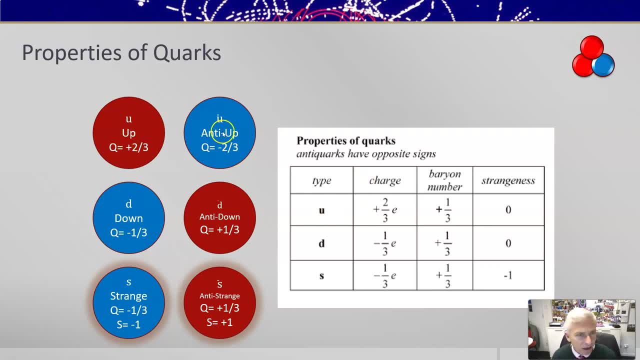 and make up the proton and neutron and an up and a down quark make up the majority of the matter in the universe. they identified some more quarks beyond the strange quark. with the strange quark we have a strangeness of minus one. strangely, an anti-strange quark has a strangeness of plus one. 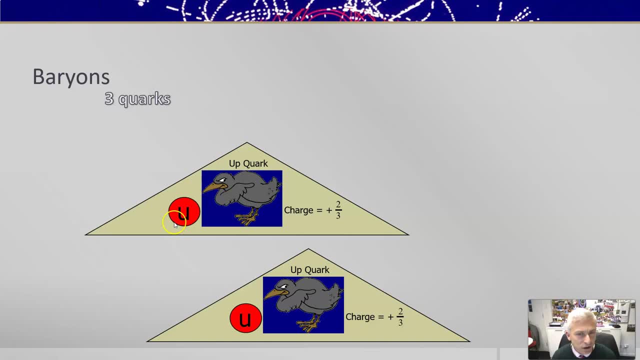 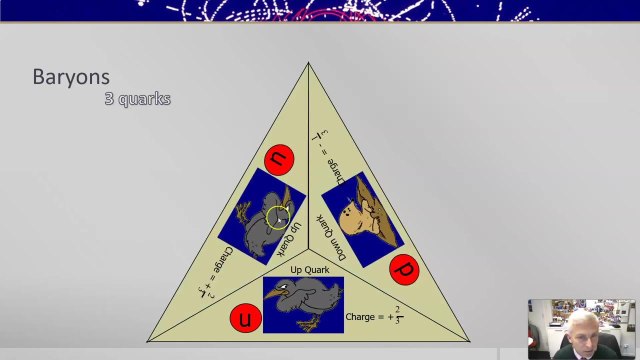 baryons consist of three quarks. now I designed these particle cards and called them so we could play particle snap at my school, and I put them as these isosceles triangles so that baryons fit together like this. then we play, snap and make a baryon, let's say an up and up and a down quark, so there's a proton or we can make. 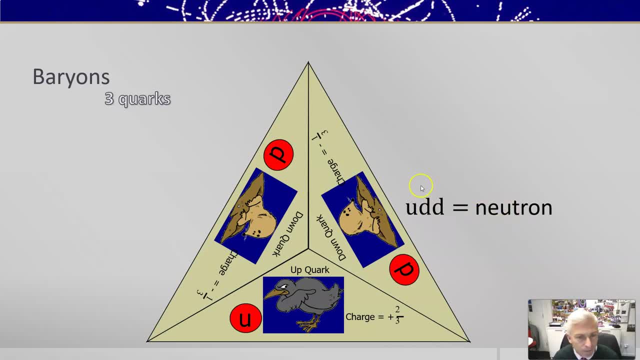 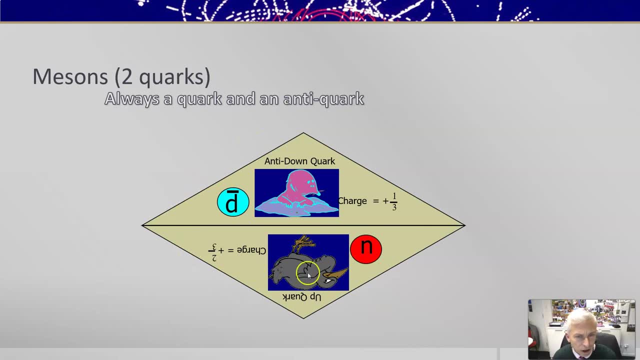 here a neutron, up, down, down as a neutron. but baryons also fit together, as these two can fit together in this shape to make a kind of kite, and that is a meson. two quarks make a meson. mesons are always a quark and an anti-quark. they don't last very long, perhaps because of this particle. 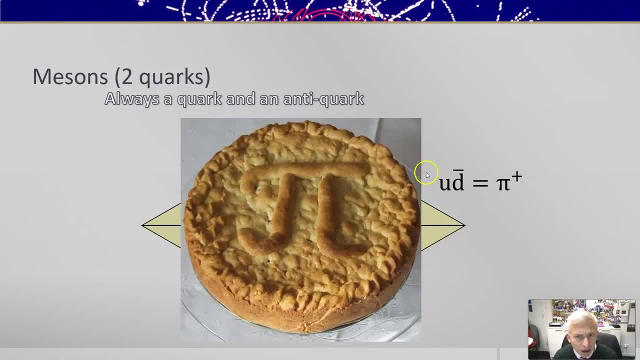 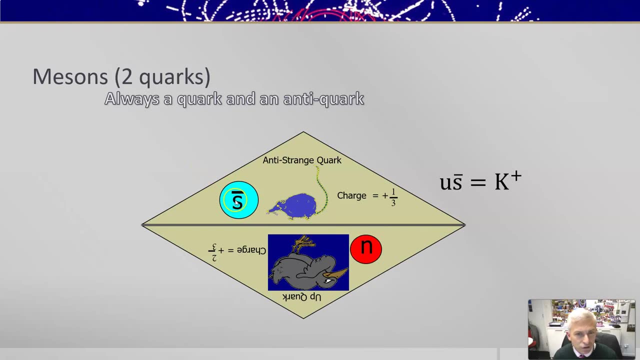 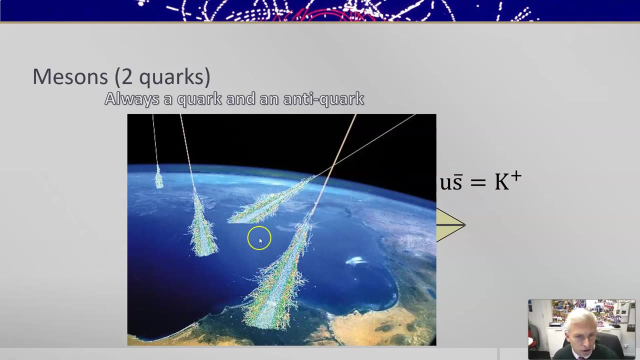 anti-particle nature, they decay and they don't last very long. this is a pion and there's a pie printed on a pie and here is a up and an anti-strange quark which makes a positive kaon. kaons can be detected in our upper atmosphere caused by cosmic ray showers and 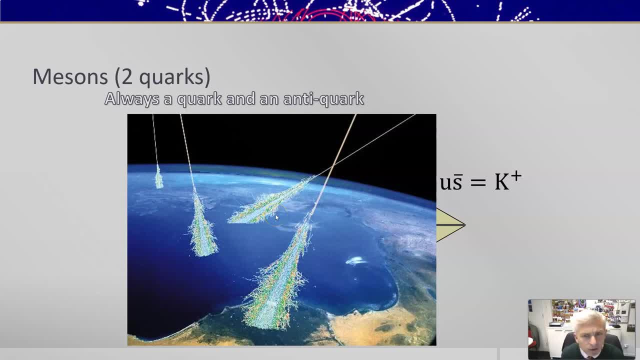 they're half, they. they have a half-life, they don't live for very long and it's actually one of the particles which give us evidence for Einstein's special relativity, because we can detect how long the kaons should live for in our atmosphere and we can detect how long the kaons should live for in. 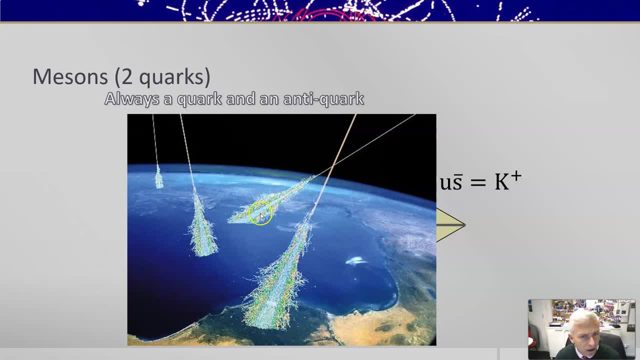 our atmosphere and we can detect how long the kaons should live for in our atmosphere, and we can. we can detect how long the kaons should live for in our upper atmosphere and we detect how many are getting down to the earth, knowing they're traveling close to the speed of. 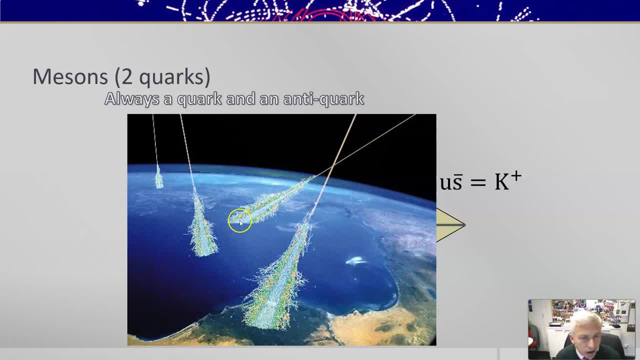 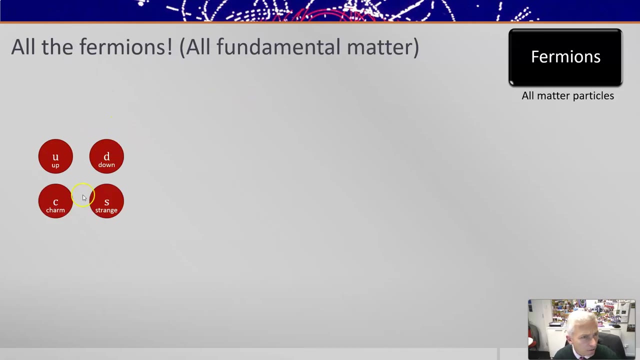 light and if they're traveling very fast, they're moving. clocks run slow. so this is one of the really good bit of evidence for Einstein's special relativity is the half-life of kaons right? so here are all the fundamental matter in the universe. we've got an up and a down, quark charm and a strange 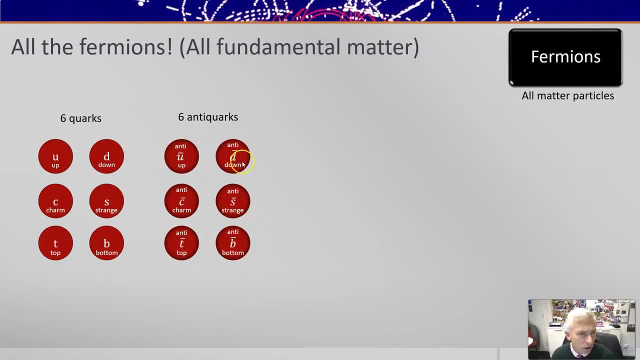 quark, top and bottom quark. so those are six quarks, and there are six anti-quarks as well. every particle has an antiparticle opposite. those are the particles of heavy stuff. and then we've got the leptons, we've got electrons, muons. 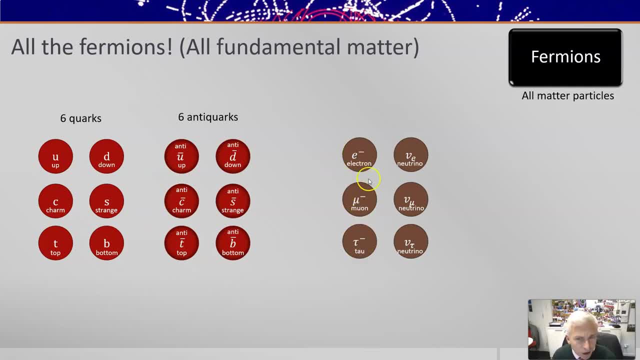 and tau. these are heavier actually and rarer, and there are neutrino equivalents of each particle. so there's a muon neutrino and a tau type neutrino. and don't forget, they're anti leptons. they have antiparticle opposites. now, if you ever meet your antiparticle, 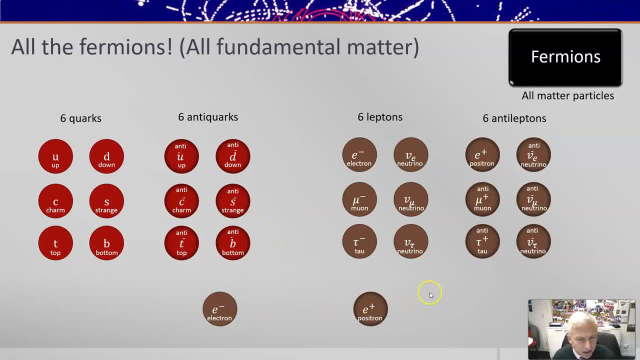 equivalent do not shake hands because matter and antimatter, when they meet, each other annihilate. so make my animation play. electron and a positron meet and they turn into energy. by e equals mc squared. now that would produce two photons. they are particles of radiation- and those photons would be 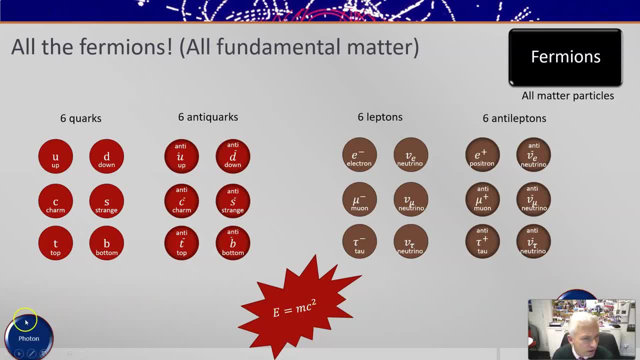 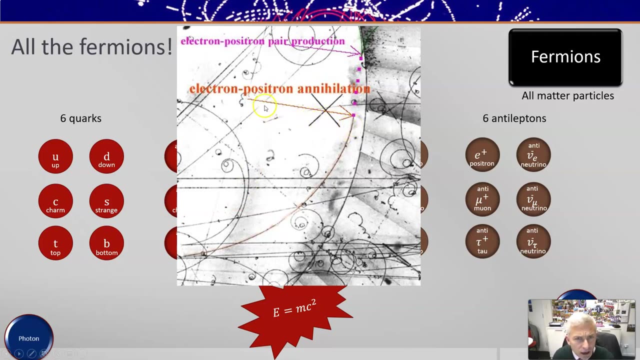 emitted. it has to be two, because we must conserve momentum. so these two must be shot off in other opposite directions, because photons, believe it or not, are also carrying momentum. so there we are. there's a crash course in particle physics are- look, here is evidence of an electron positron annihilation. so here, 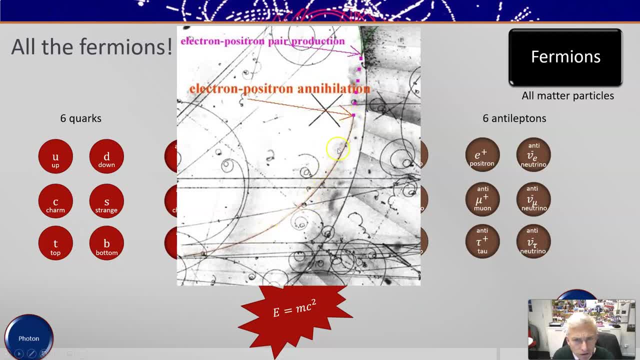 is a particle track of a moving positron. we know it's a positron because of the radius of curvature in the direction in which it curves in the magnetic field, and at this point it is annihilated. it is turned into radiation. the dotted track shows the radiation traveled along here and here is evidence that it is. 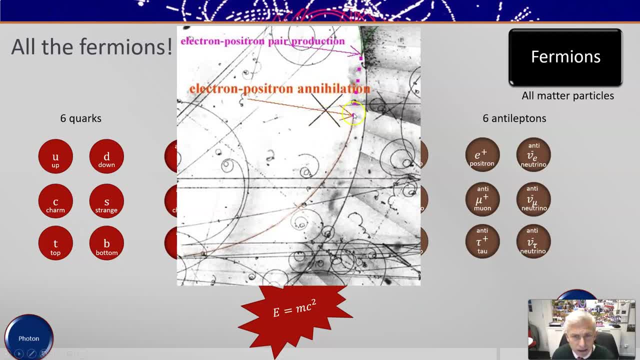 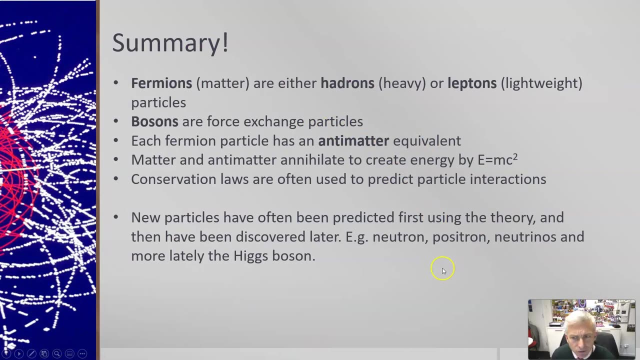 is annihilated when it is hit. a stationary electron, probably in the matter here and in whatever gas or liquid it's in. and here we've made a positron and an electron, a pair. so matter into energy here and energy into matter here. here's a summary of the kind of things you've